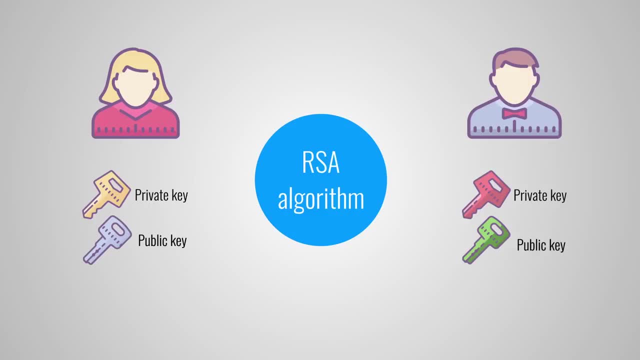 for doing this is by using the RSA algorithm. This algorithm will generate a public and private key that are mathematically linked to each other. Public keys can be used to encrypt data and only the matching private key can be used to decrypt it, Even though the keys are linked together. 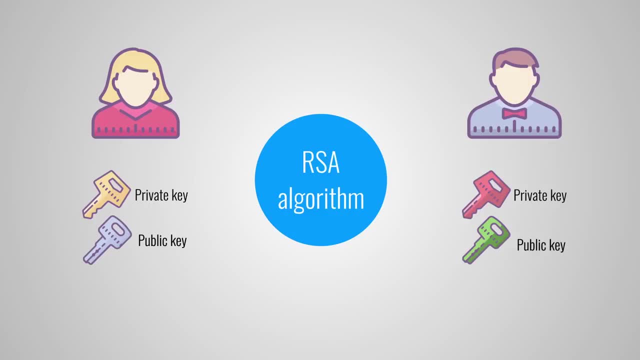 they cannot be derived from each other. In other words, if you know someone's public key, you cannot derive his private key. If we retake our mailbox example, then the mailbox's address would be the public key, something that everyone is allowed to know. 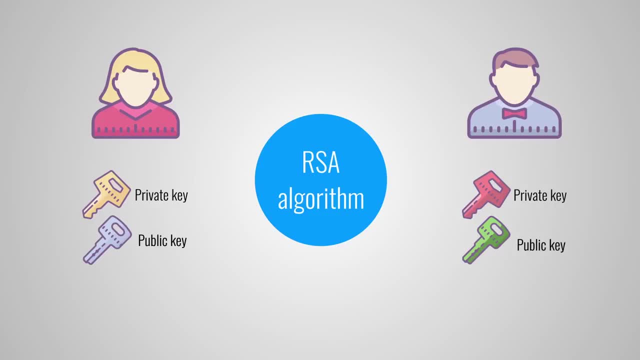 The owner of the mailbox is the only one who has the private key, and that is needed to open up the mailbox. Let's now take a look at how Alice and Bob can use asymmetric encryption to communicate securely with each other. They start by exchanging their public keys. 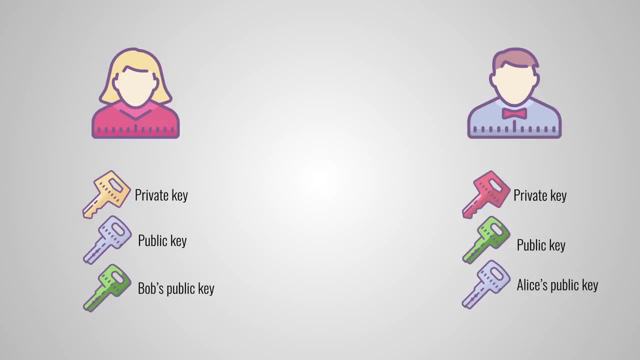 Bob gives his public key to Alice and Alice gives her public key to Bob. Now Alice can send her sensitive document again. She takes the document and encrypts it with Bob's public key. She then sends the file to Bob, who uses his private key to unlock the document and read it. 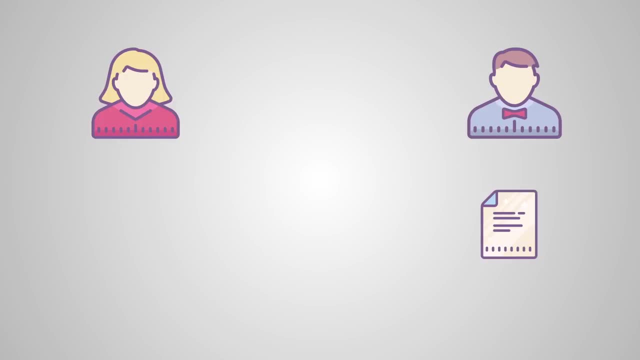 Because they use asymmetric encryption, only Bob is able to decrypt the message. Not even Alice can decrypt it because she doesn't have Bob's private key. The strength and security of the asymmetric encryption now relies on Alice and Bob to keep their private keys well protected If an attacker 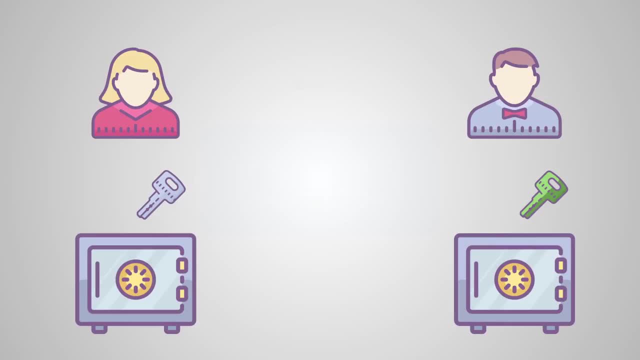 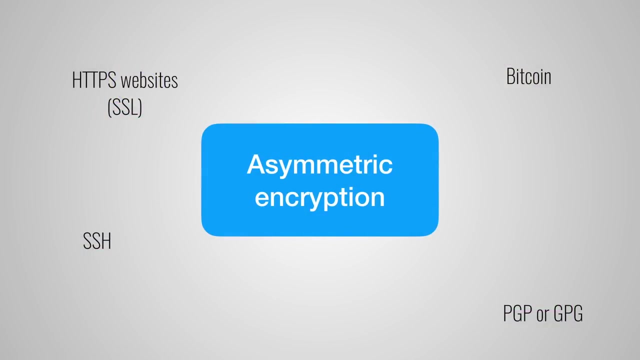 steals Alice's private key, it can be used to decrypt all messages that are intended for Alice. However, the attacker cannot decrypt messages that were sent by Alice, because that requires Bob's private key. Asymmetric encryption is used in a lot of places where security really matters. You might not be. 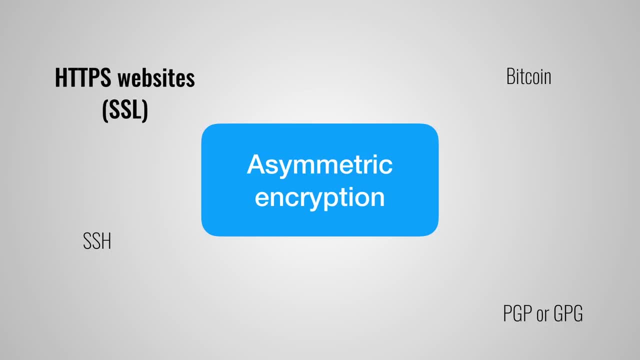 aware of it, but every time you visit a secure website via https, you're actually using asymmetric encryption. It's also being used to securely send emails with the PGP protocol. And one last example: Bitcoin also uses asymmetric encryption to make sure that only the owner of a money wallet can withdraw or transfer money from it.